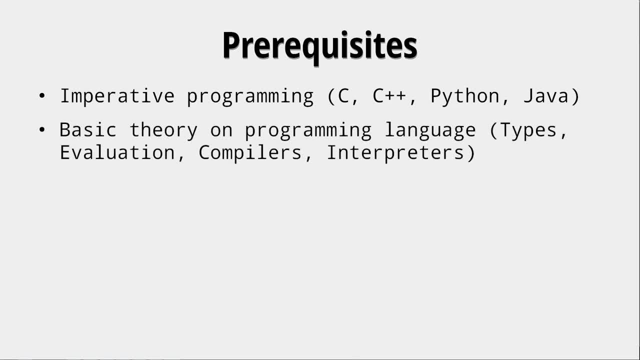 theory on programming languages. So you should know what types are and how they work, how evaluation of expressions work and what the difference between a compiler and an interpreter is. for example, You should have the Haskell toolchain installed, So GHC, GHCI and Cabal. 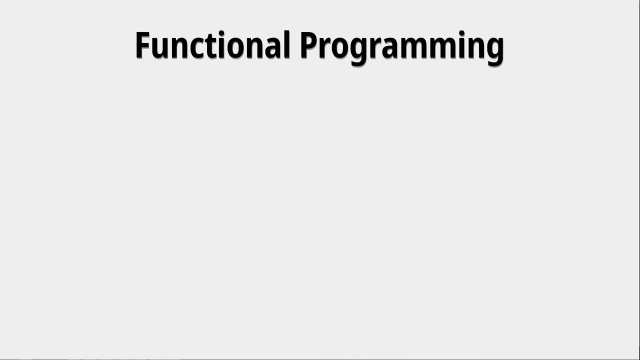 should all be installed on your computer. So okay, let's look at what functional programming actually is and what it means to have a functional program. Well, in functional programming, and especially in Haskell, we are interested in pure functions, meaning functions in the mathematical definition. that 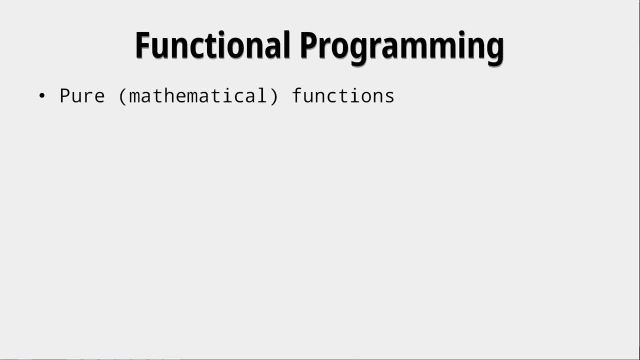 they have some input, some arguments, and then have a result and nothing else. We are also interested in immutable data, meaning that our data types, whatever they might be, cannot be changed in place. Those two attributes- pure functions and immutable data- lead to no or less. 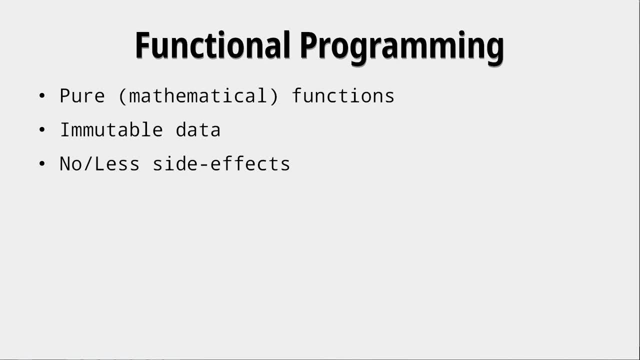 side effects. Side effects are especially dangerous and are very hard to verify. Their absence is very hard to verify, which is why we don't really want them. Functional programming in general is more declarative, or is declarative instead of imperative, and the difference. 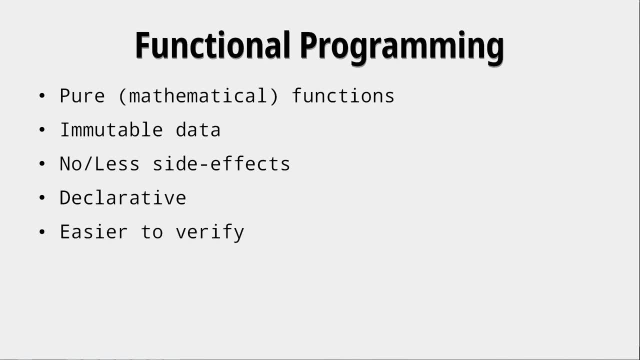 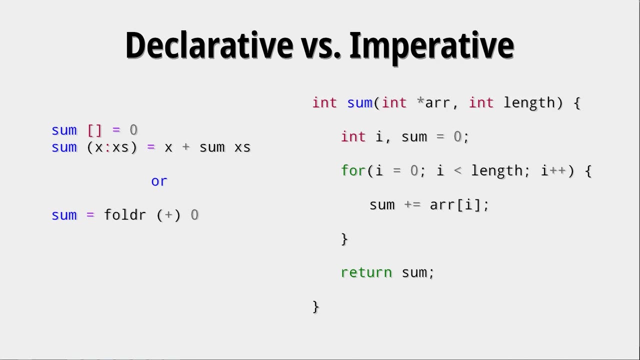 we will highlight in just a second. Functional programs in general are easier to verify, and that is a huge part of functional programming, since we can actually mathematically prove the correctness of our algorithms. So let's look at the difference between a declarative and an imperative approach when 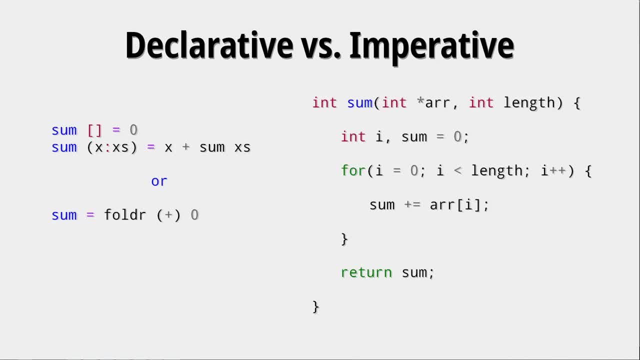 comparing them on a function that computes the sum of an array or list of numbers. So in the imperative approach on the right we can see that for each step that we do we tell the program what to do. So we say: set the sum to zero, then set i to zero, then 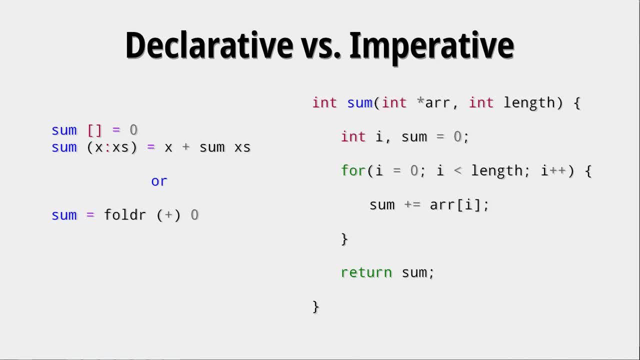 iterate until a certain condition is met and then set the sum to zero and then set i to zero, and then iterate until a certain condition is met and then set i to zero, and then iterate until a certain condition is met and take every single value of that. 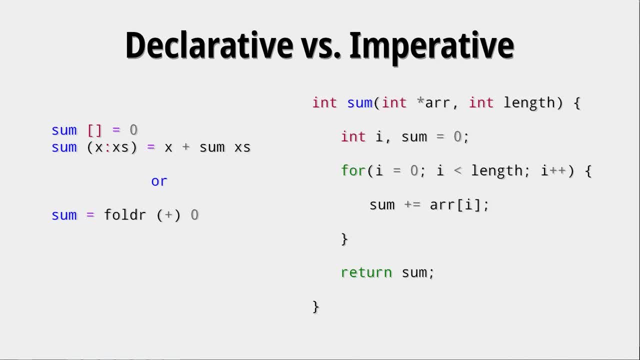 array, which, of course, is dependent on this. i index and then add it to the sum And after that, of course, return the sum. So what we are doing is not give a definition of what it means to be a sum or what a sum actually is. we just describe an algorithm that can. 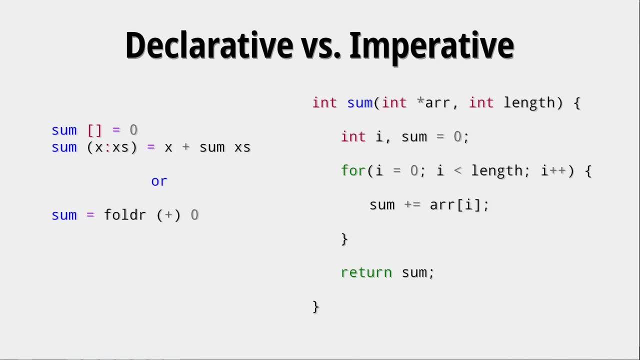 produce a sum. Now, in the declarative approach we actually define, or sort of define, what it means to have a sum. So we say that a sum of an empty list is just zero and a sum with a list with at least one element x is that element x plus. 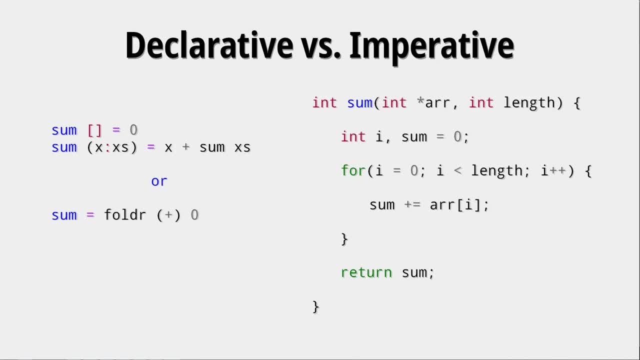 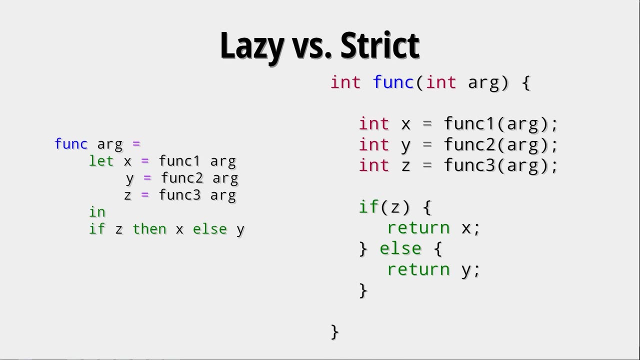 whatever the rest of the sum is. Now, using some fancy tricks like partial function application and the folding function, we can have a much shorter function definition. but what that actually means we will learn later. So one very important thing of Haskell is that it's lazy evaluated, Lazy evaluation. 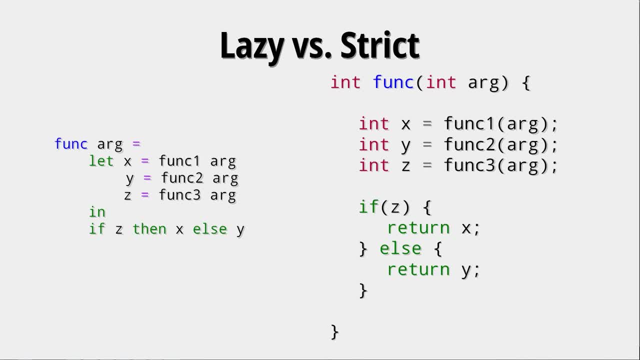 is something you need to get your head around when working in Haskell. So let's look at something that is strictly evaluated. Let's assume that the functions func1,, func2, and func3 all take one year to finish In a strictly evaluated language like, for example, C or Java. 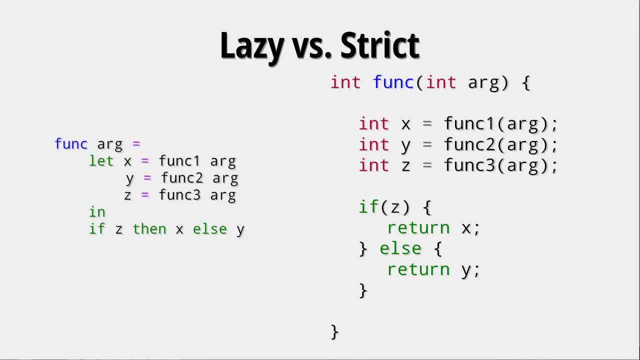 the example on the right would take three years to finish. In a strictly evaluated language like, for example, C or Java, the example on the right would take three years to finish Because of course we first evaluate func1, that will take a year. then we evaluate func2,. 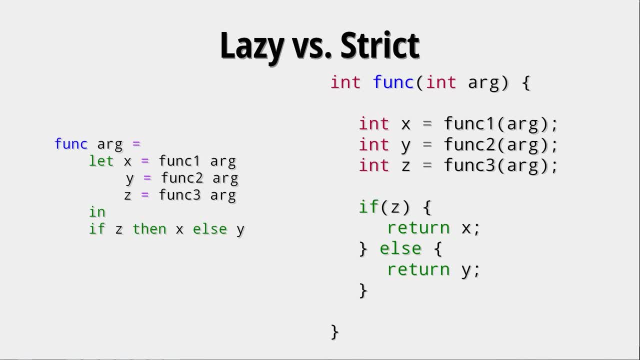 and then func3.. After that we do this if-then-else, which probably won't take that long. So the whole function takes three years to finish. How does it work in Haskell? Well, if Haskell is lazy evaluated- which it is- then it works like this: We have the definitions x, y 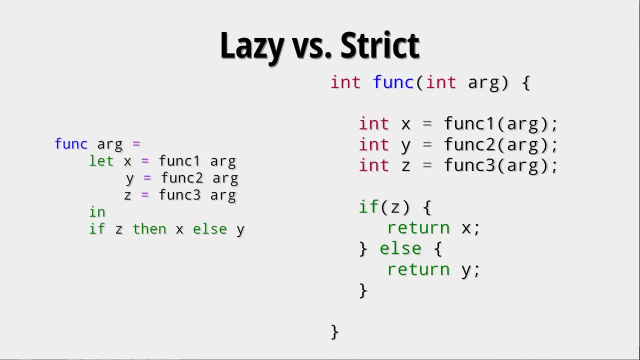 and z on the left And as the result of certain functions. Now they are not evaluated right when they occur in the code. because they don't have to right now, Because Haskell looks at what has to be evaluated in order to get the result and it first observes that: yeah, well, we need. 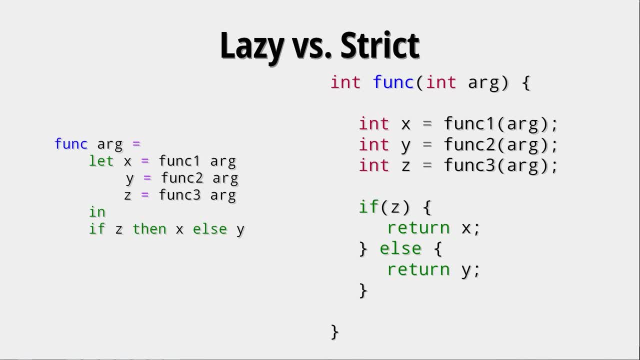 z, because otherwise we can't do this if-then-else. So z is evaluated, which takes one year, And then we either evaluate x or y, which takes another year. algorithm will only take two years. so i mean, that is some performance improvement, i guess.